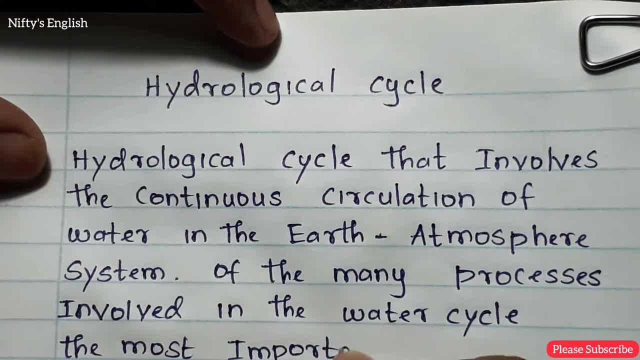 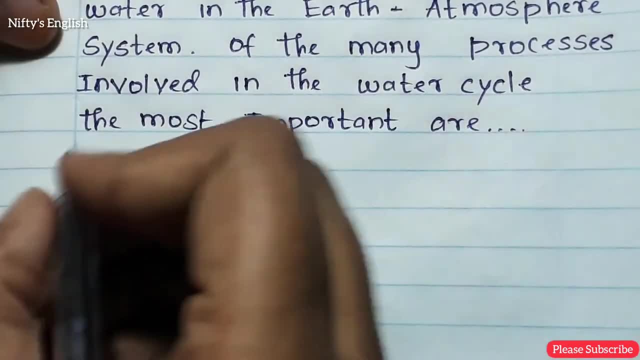 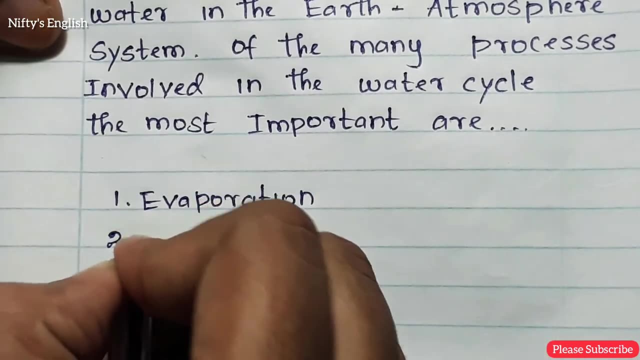 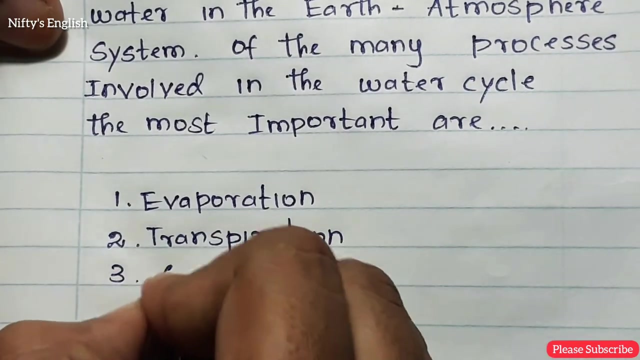 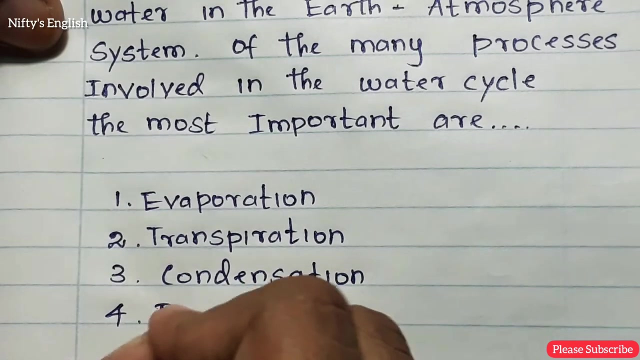 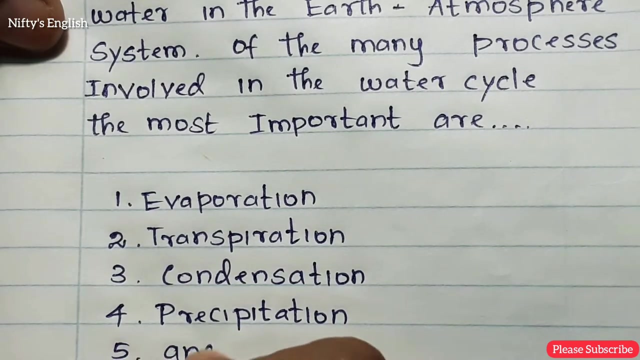 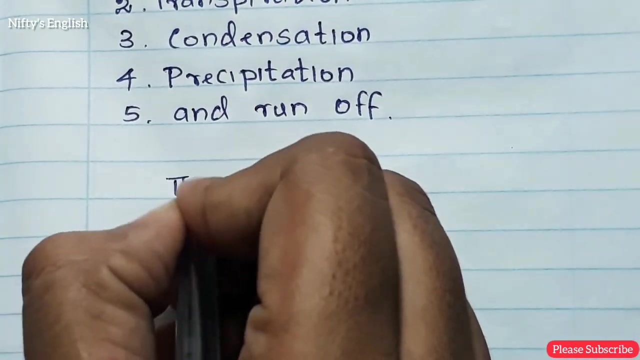 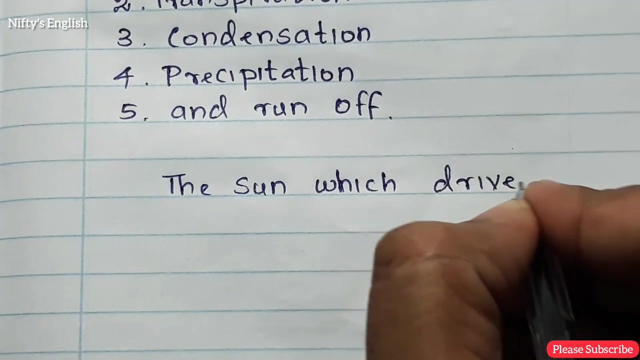 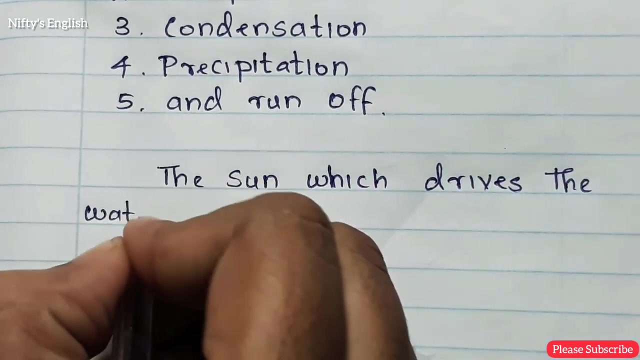 the most important are the most important are. the most important are: number one, number one- evaporation. evaporation Number 2, Transfusion- Number 3,. Contentiation- Number 4, Precipitation- Number 5, and Runoff Number 4,. The Sun, which drives the water circle, heats water in oceans and seas. 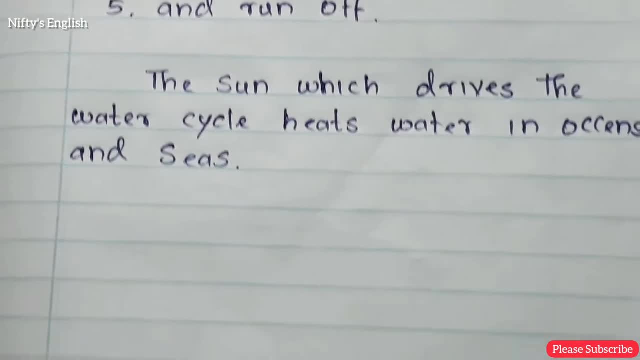 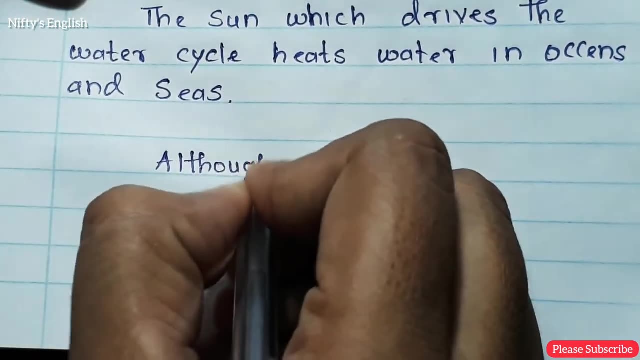 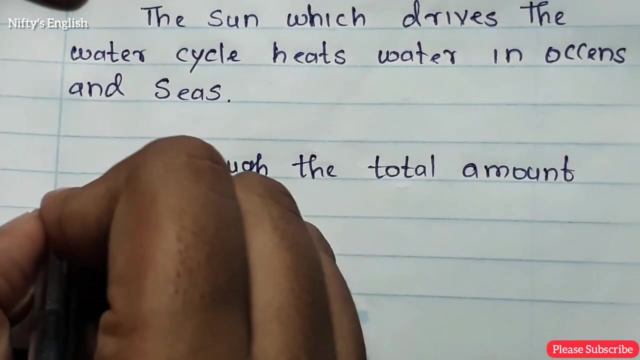 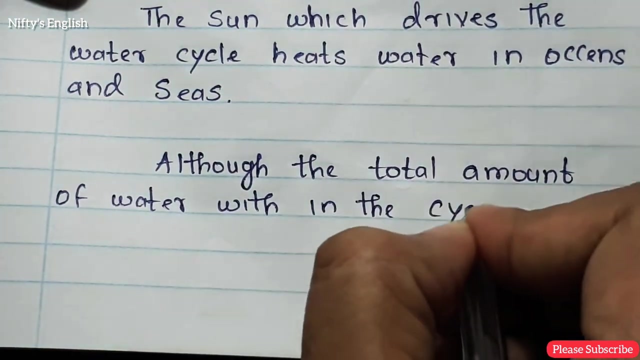 Number 5, Although the total amount of water within the circle remains essentially constant. Number 6, The Sun, which drives the water circle, heats water in oceans and seas. Number 7, The Sun, which drives the water circle heats water in oceans and seas. 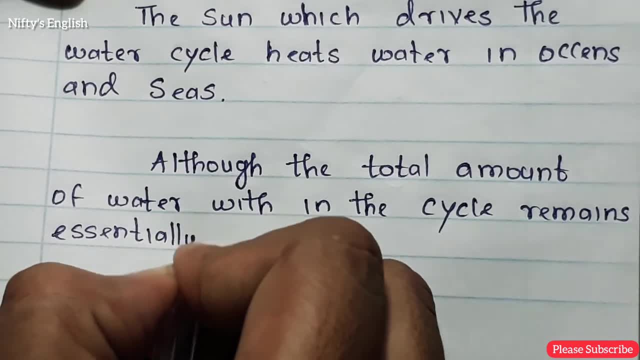 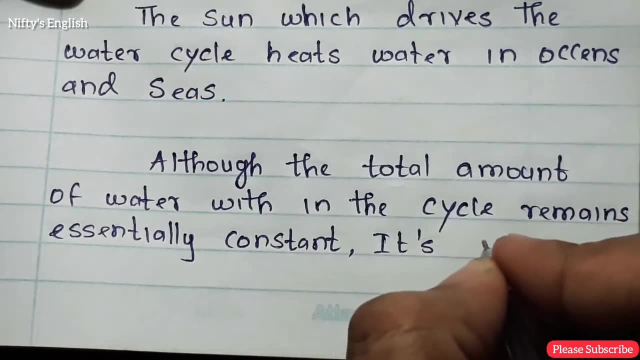 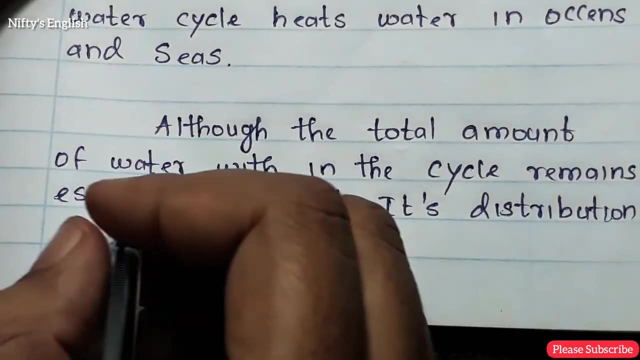 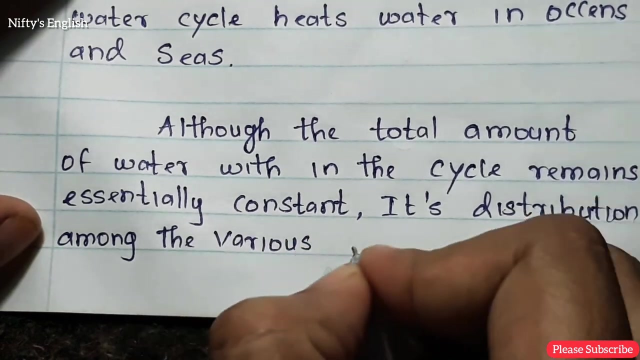 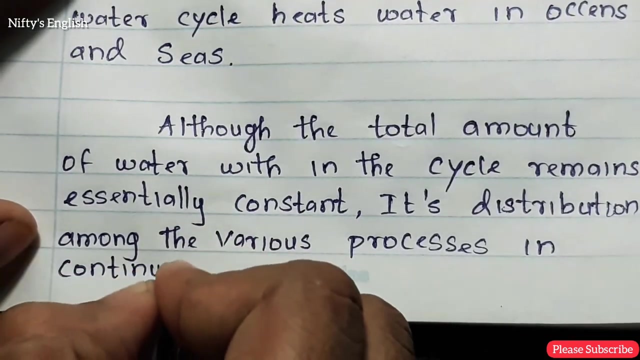 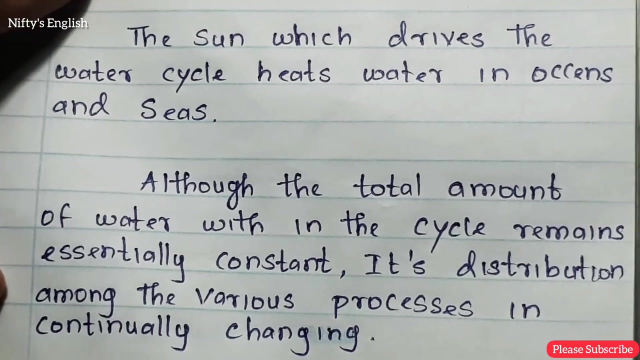 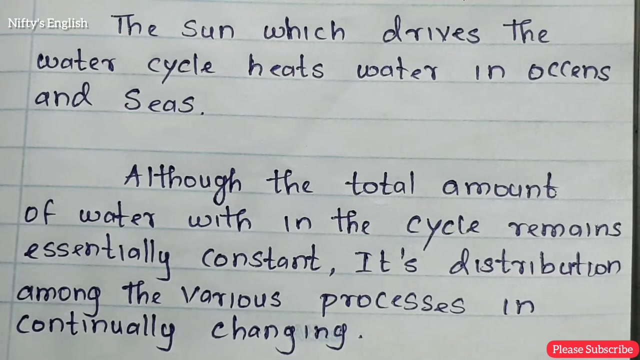 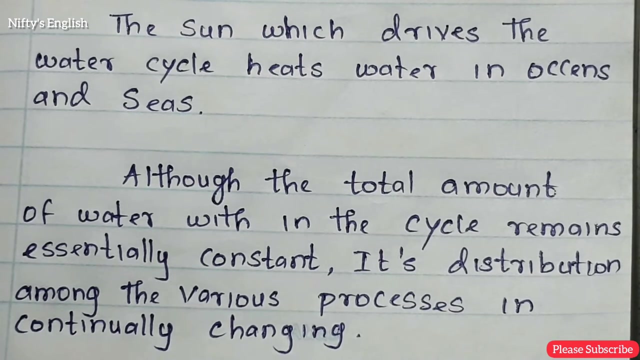 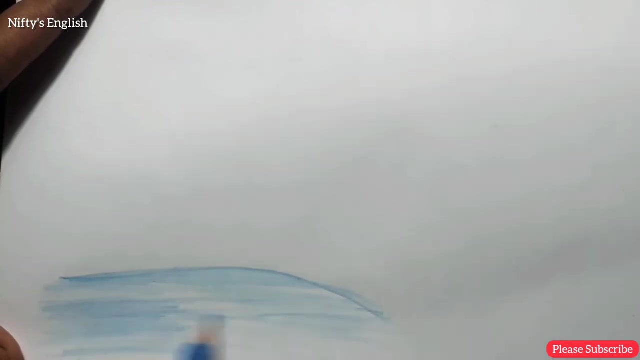 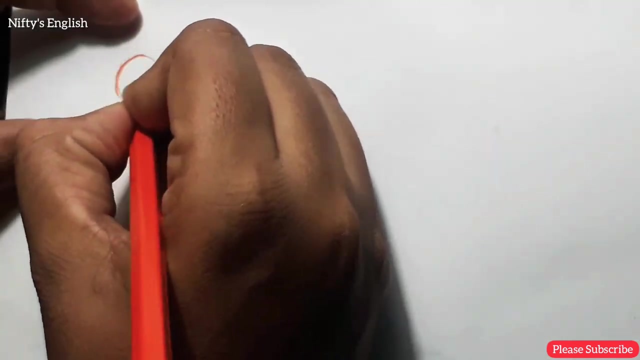 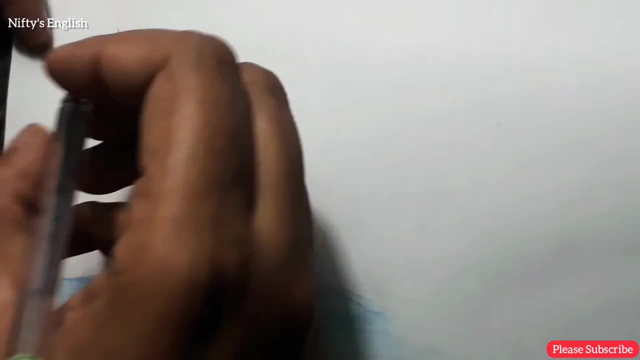 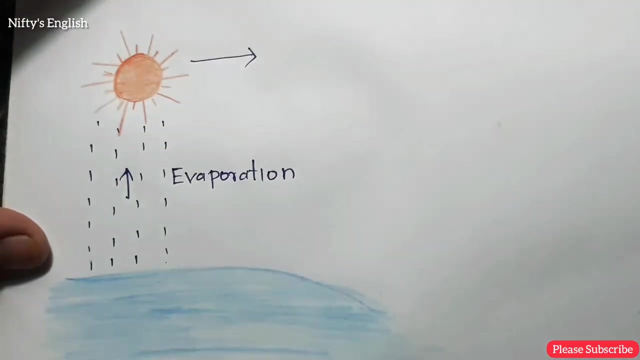 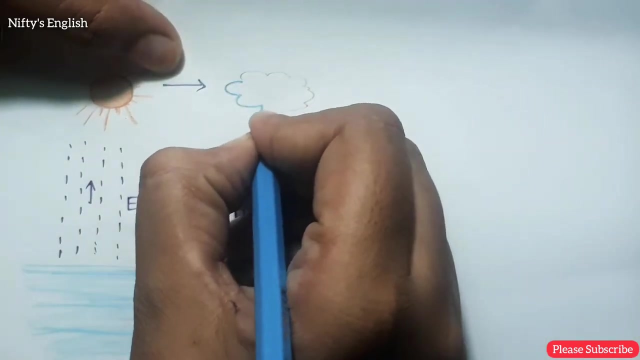 Number 8, The Sun, which drives the water circle, heats water in oceans and seas. Number 9, The Sun which drives the water circle heats water in oceans and seas. Number 10, The Sun which drives the water circle heats water in oceans and seas. 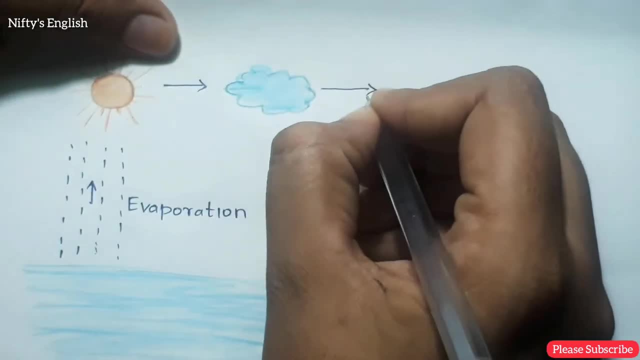 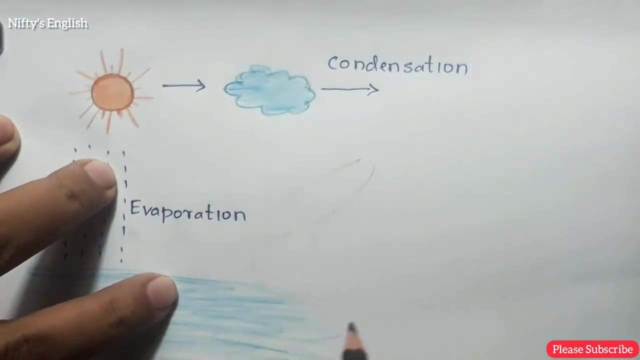 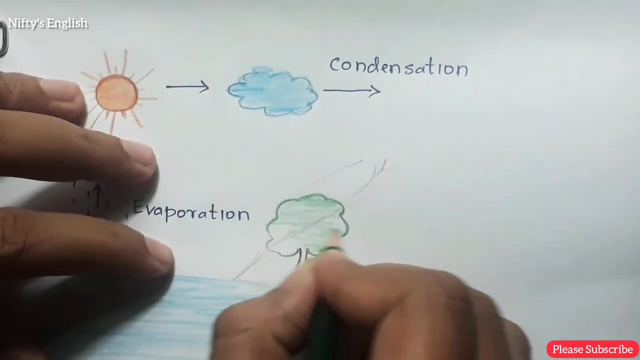 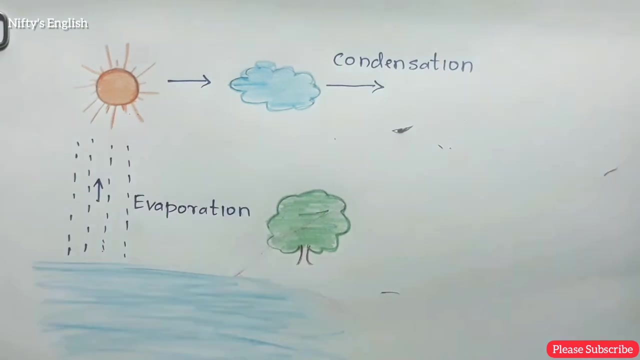 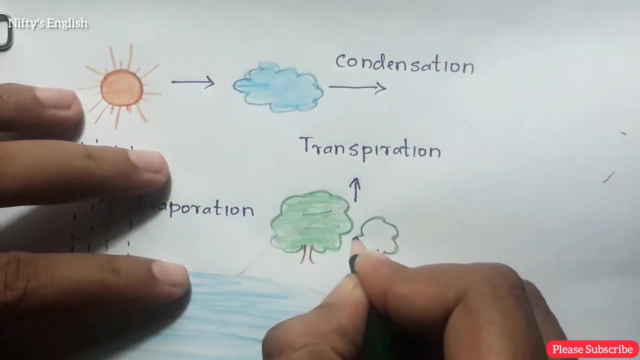 Okay. Second one is condensation. Condensation is the process of a gas changing to a liquid in the water cycle. Water vapor in the atmosphere condenses and become liquid, Okay. Another one is transpiration. Transpiration is another important part of the water cycle. Transpiration is the process of water vapor being released from plants and soil. 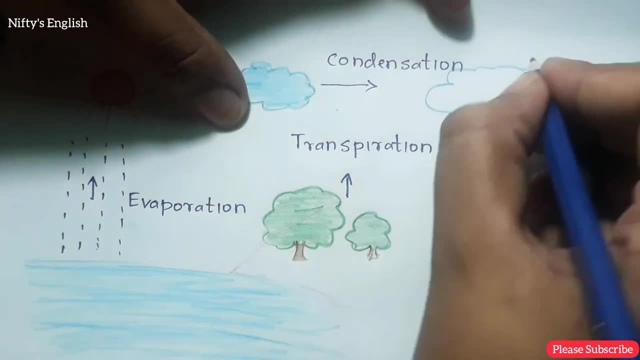 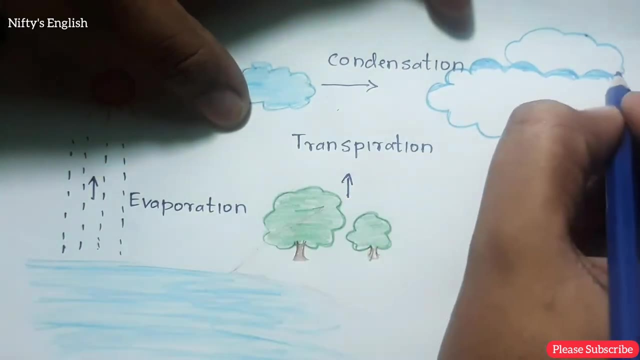 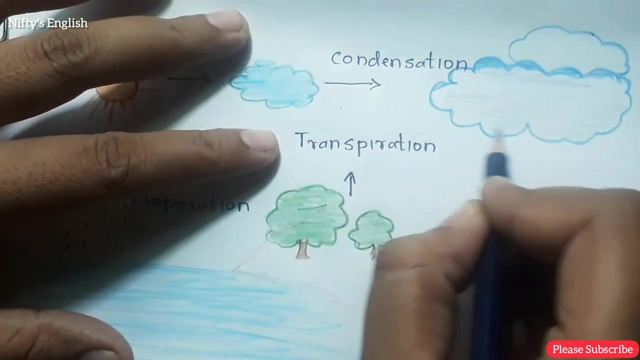 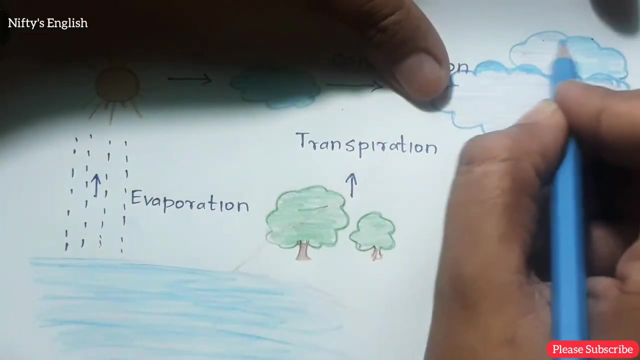 The one of the major process of water cycle: precipitation. as the case with evaporation and contention, Again precipitation is a process. Precipitation describes any liquid or solid water that falls to earth as a result of contention In the atmosphere. precipitation includes rain, snow and hail. 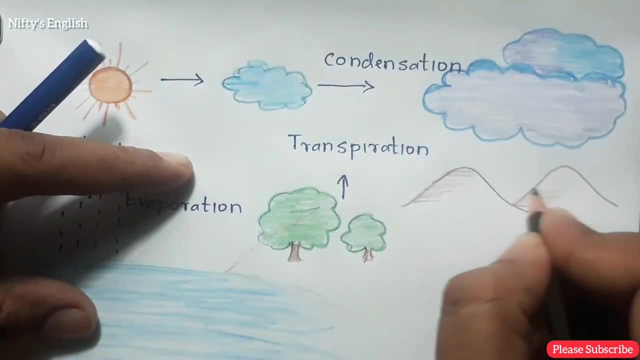 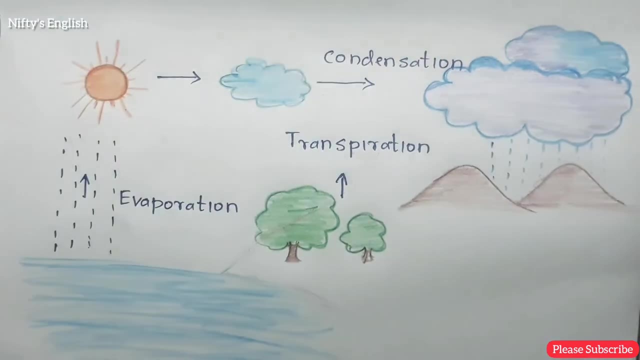 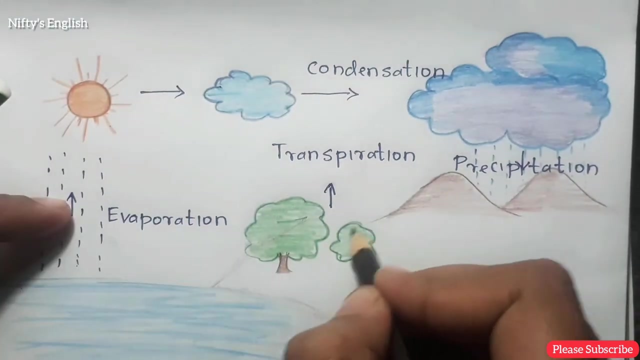 Precipitation is one of many ways water is cycled from the atmosphere to the earth or ship. Again. precipitation is another important part of the water cycle. Transpiration is another important part of the water cycle. Evaporation, contention and precipitation are important parts of the water cycle. However, they are not the only ones. 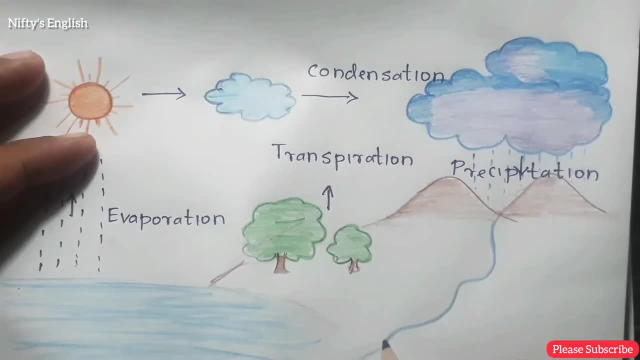 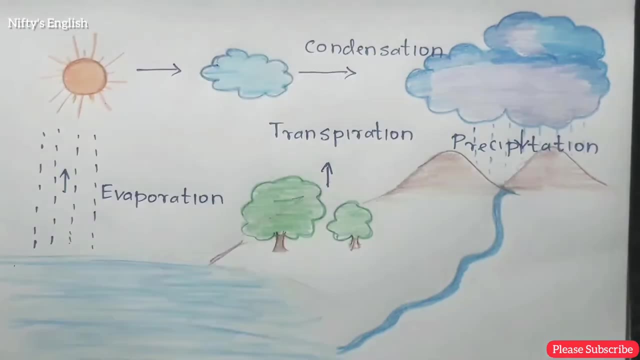 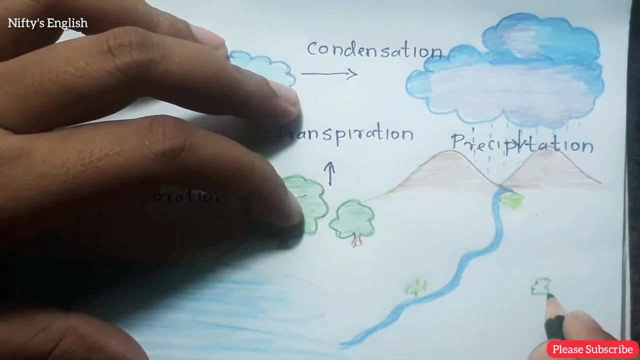 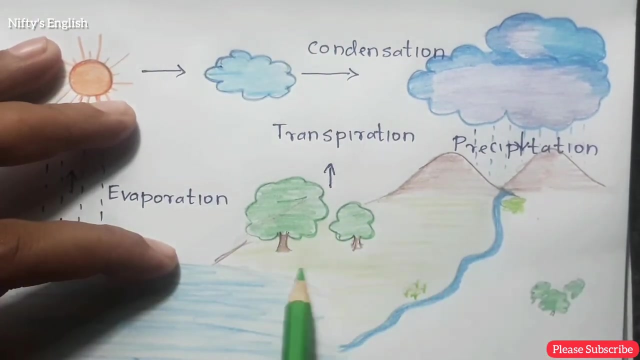 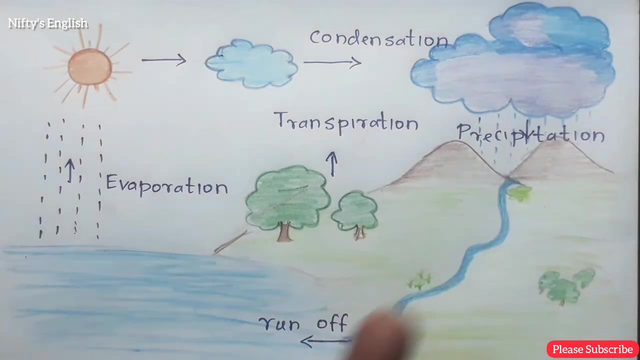 Another process of water cycle is transpiration and runoff. Next one is runoff, Next one is runoff, Next one is runoff. For instance, it describes a variety of ways liquid water moves across land. snow melt, for example, is an important type of runoff, produced as snow or glaciers melt and form streams or pools. it's a circle. 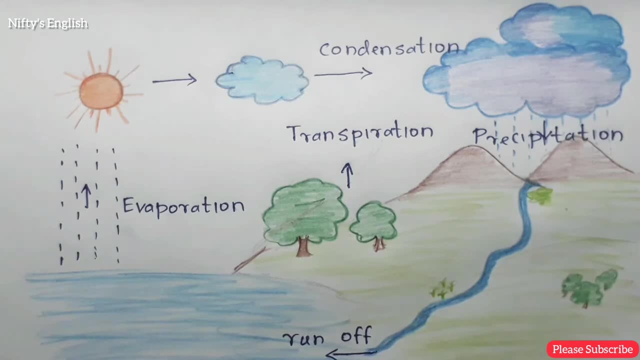 a vibration transformation contentious, and precipitation and runoff. and again, a vibration transformation contentious, and precipitation and runoff. okay, that's it. please subscribe and press the bell icon. thank you, keep supporting us. have a great day, all of you.